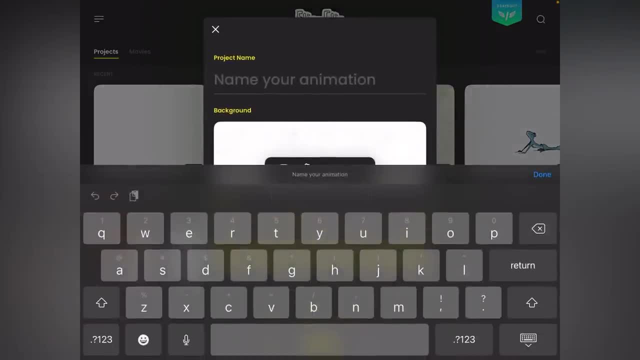 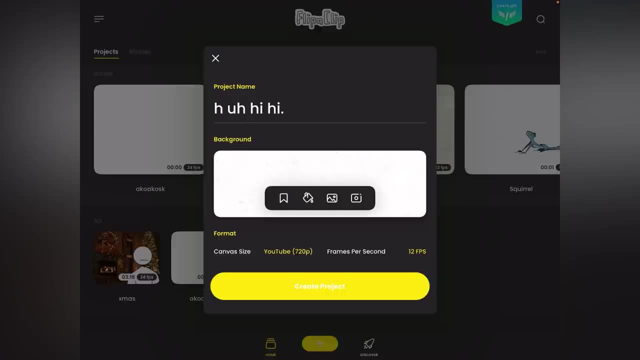 Now we get to customize the project variables. Step one: give it a great name. Wow, that's, uh, that's something. The background is automatically white now, but you can choose from a set of backdrops or import your own. 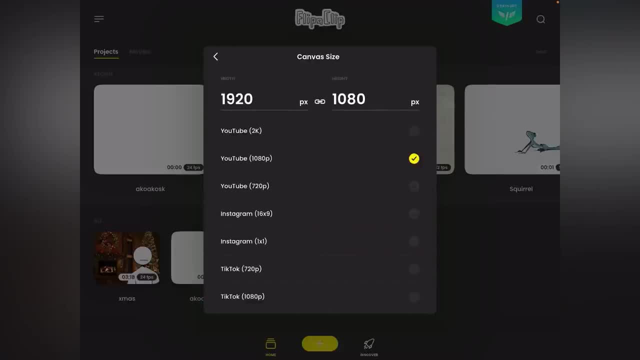 For canvas size. I used 1080p For my YouTube videos, so I'm gonna go ahead and click that. one FPS or frames per second basically means how choppy or smooth the animation will look, based on the amount of frames in the second of animation. 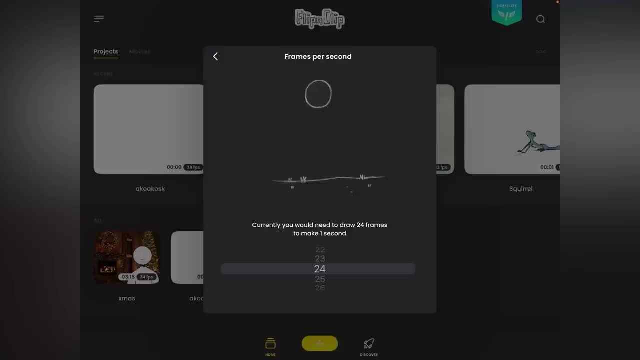 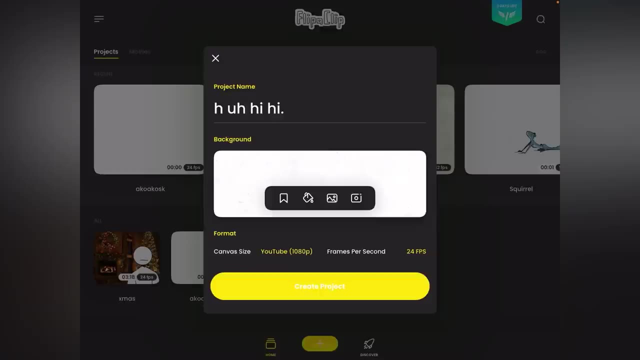 I usually use 24 FPS, as do most YouTube animators, but feel free to go lower or higher. The higher the FPS, the more frames you'll have to draw, but the better it'll look in the end. Alright, we are all set. now Go ahead and press create project. and now we are in the animation interface. 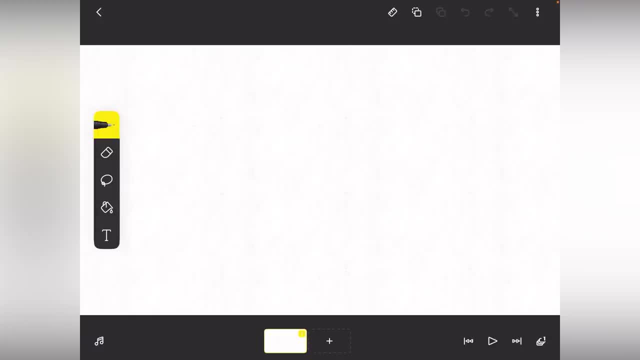 I'll start by explaining the tools on the left hand side. This here is the drawing tool menu. I use the pen, aka the default sketching tool, but by clicking on it you can adjust size, opacity. wait, I had to put that. 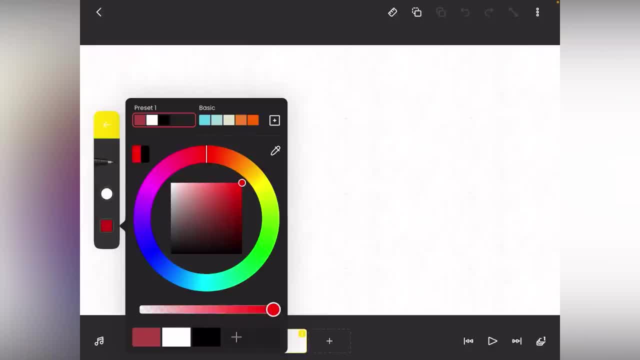 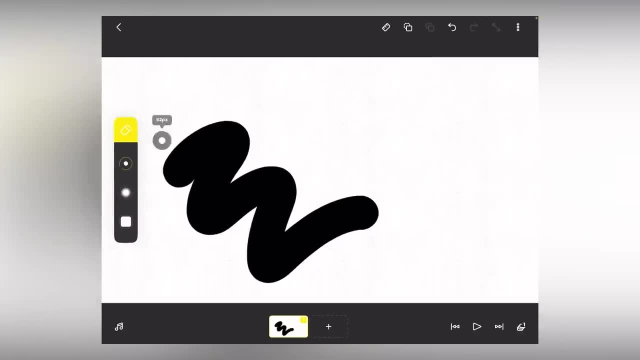 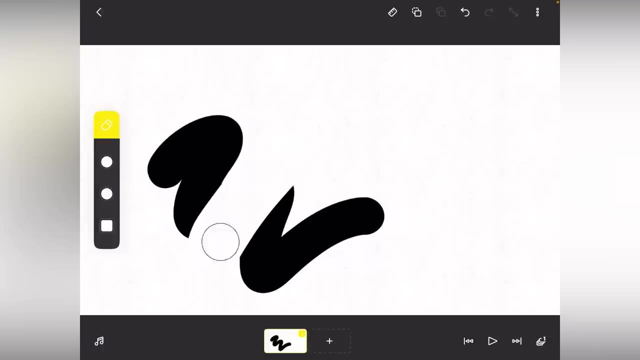 and color Bam. That's a thick line. Next, eraser for getting rid of life's mistakes. Don't bother trying it on yourself, I already have. You can adjust the feathering opacity and size of the eraser tool, similar to the sketch tools. 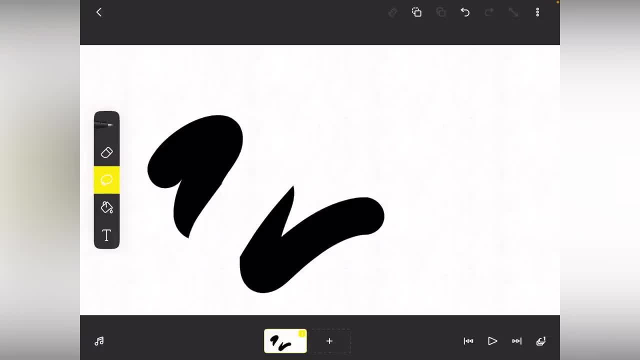 Next is the selection tool. If you have a part of a drawing you want to move or change or something, you just draw a selection around it and then you can liquefy it to your discretion. Below that is the fill tool, or paint bucket. It fills in areas with a solid color. 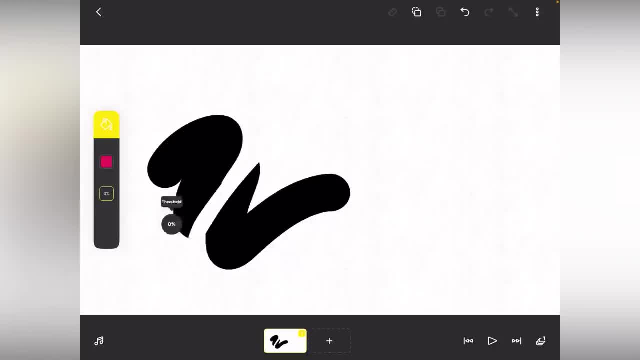 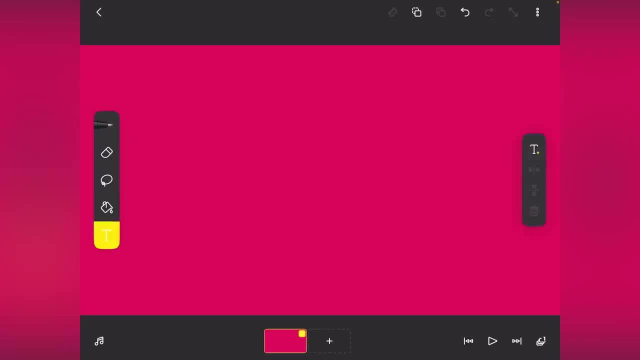 Now you can adjust the full threshold. so if there are little gaps that you don't feel like correcting, lower the threshold and the full will stay inside the lines instead of covering the entire friggin canvas. Finally, we have the text tool. Pretty simple, just. 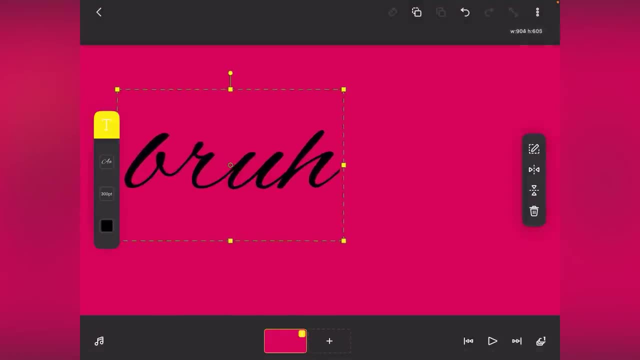 enter some text. That's basically it. You can pick the font color and size, which is pretty cool. Wow, Up here we have the ruler tool. You can choose from a line ruler, a circle ruler or a rectangular ruler. 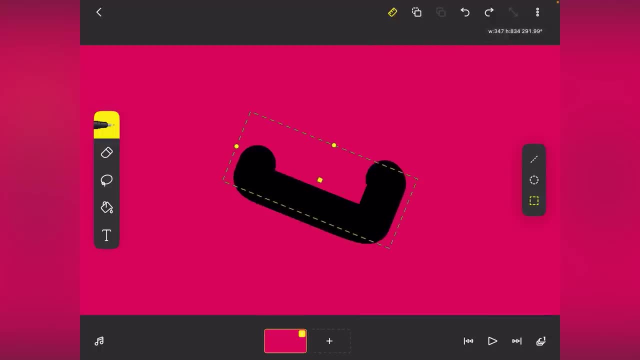 You can adjust each of them to your needs, and all you need to do is draw while it's activated and your lines will be as straight or as curvy as you need. Next, we have the copy and paste buttons. You can copy and paste frames as well as selections. 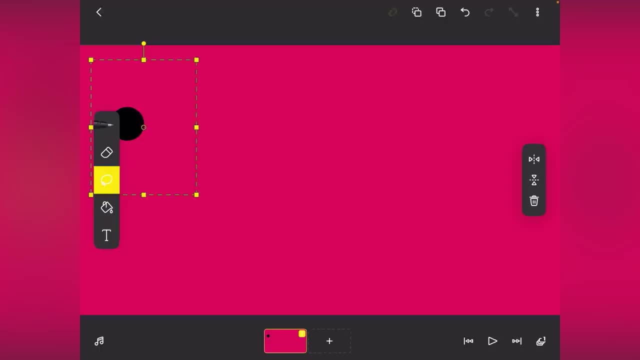 so if I went and did a little scribble and I wanted to only copy the scribble, I would do that. Whoa, there's two of them. Here are the undo and redo buttons. If you don't know what that does, I am seriously concerned. 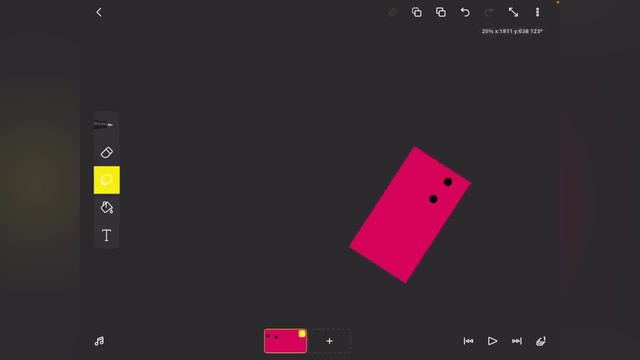 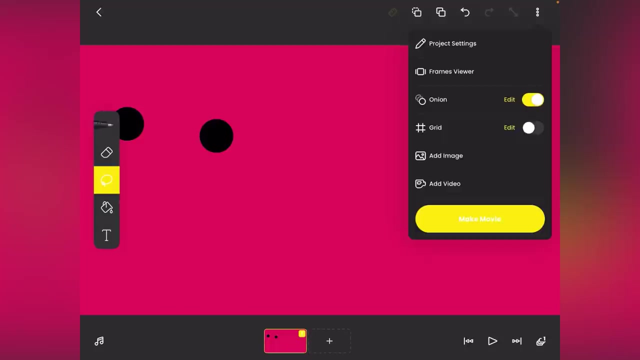 The reset view button. If you accidentally made your canvas all weird by zooming out or tilting it, press this to go back to the original location. Next, the ever so ominous three dots. These are kinda like the settings. Here you can edit project settings. view all the frames. 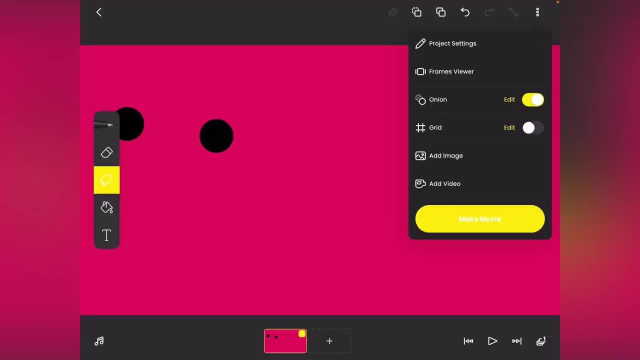 and mass duplicate or delete them. edit onion skin. edit the drawing grid, add an image or add a video. And no onion skin isn't actual onion skin. that would be really weird. Also, when you're all done with your project. 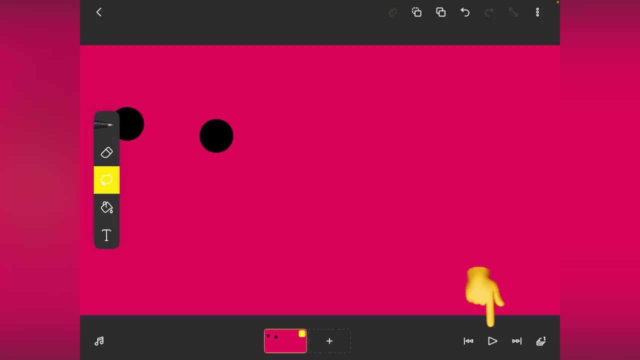 press make movie to export it. Bottom right we have the skip to beginning and end buttons, as well as the play button. Here's the layer manager where you can- I don't know- manage layers. you know, add them, move them around. 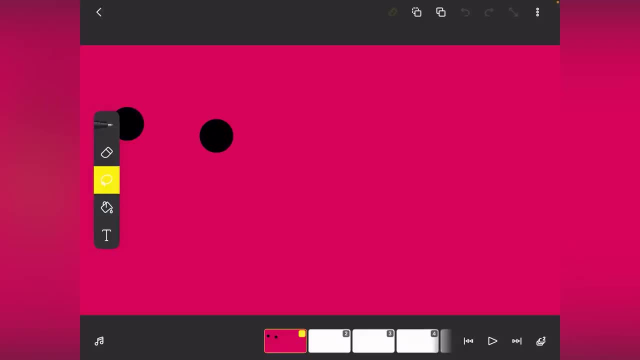 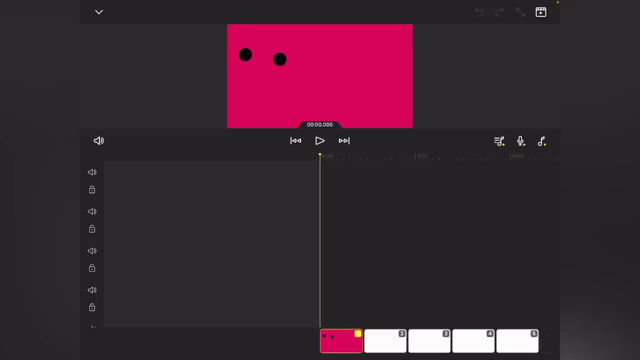 delete them and stuff. Wow, Bottom left is the sound window. It contains a bunch of different audio tracks to put sound clips in. For example, if you wanted to import an audio file, you would press the button on the right here and import the file. 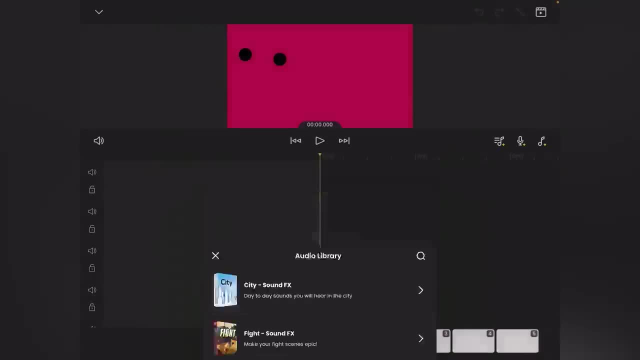 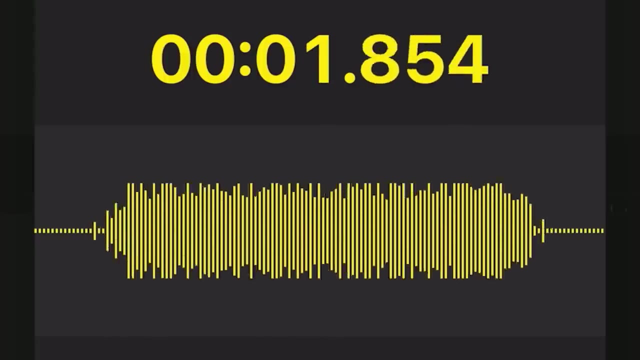 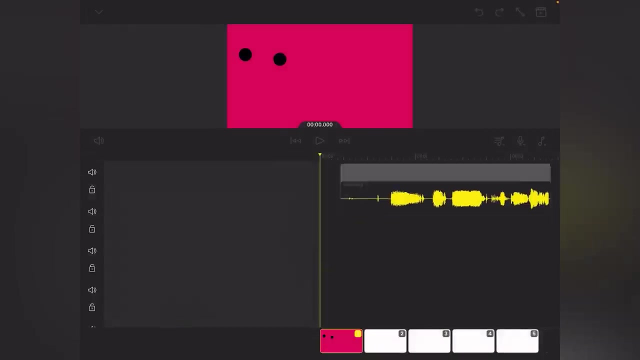 There's also an audio library and an audio recorder, Which I am going to use right now. Okay, um, um, I like chicken, Um, I like chicken. Oh, wow, I love that. Okay, so we're gonna drag it to any track, as suggested. 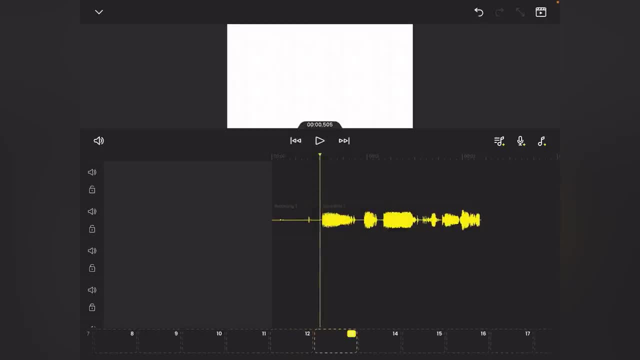 I'm gonna trim off the beginning bit because no one needs that. And we have: I like chicken, Chicken. And then we have a great audio here. Um, I like chicken, I like. that's great. okay. Now I am going to try to animate. 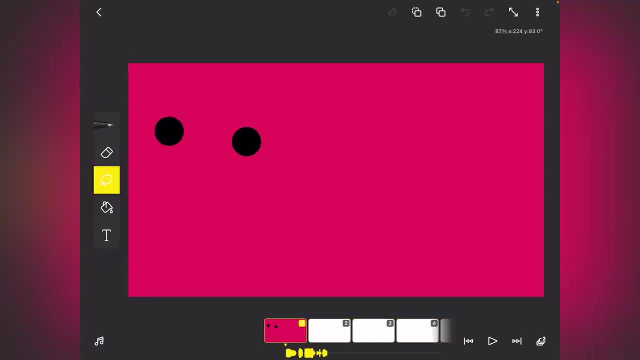 that for you guys. First of all, delete whatever this is Bam. what, Oh oh, wrong layer. Yeah, see, I'm such a pro at flip a clip- I know, I know how to use it so well. 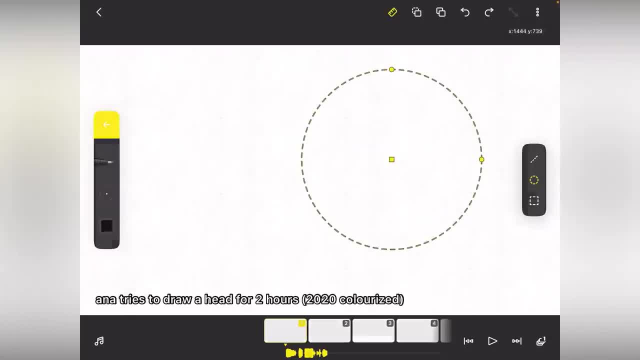 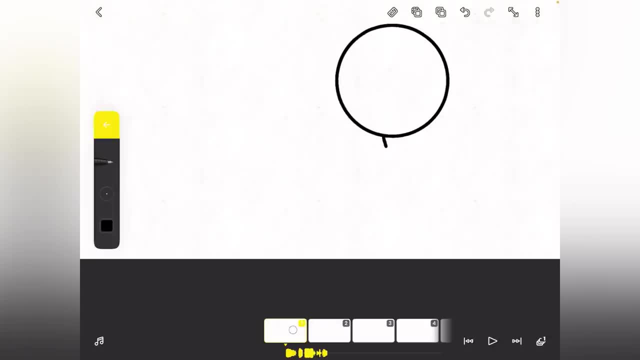 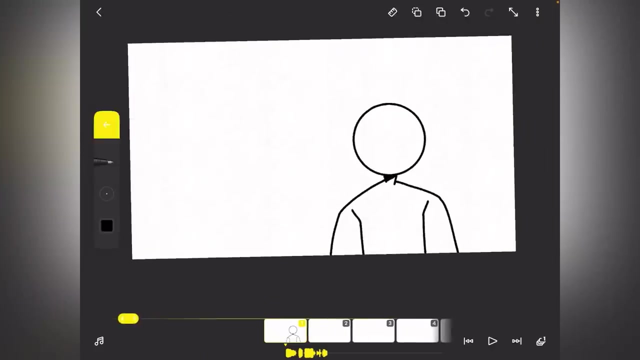 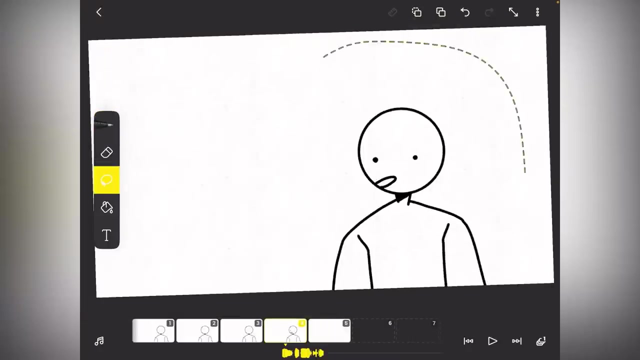 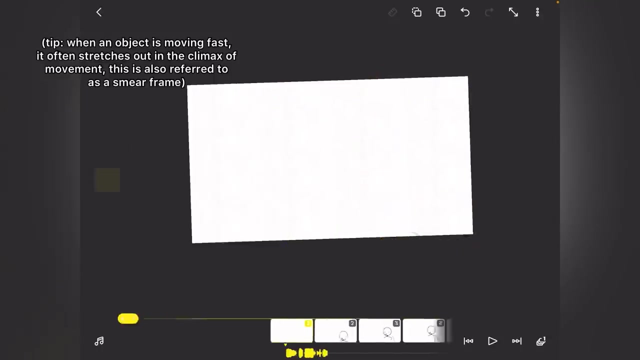 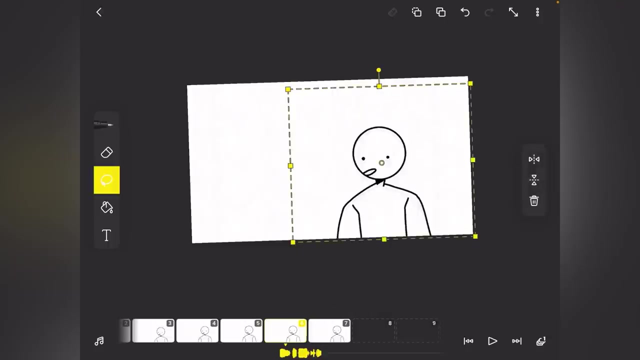 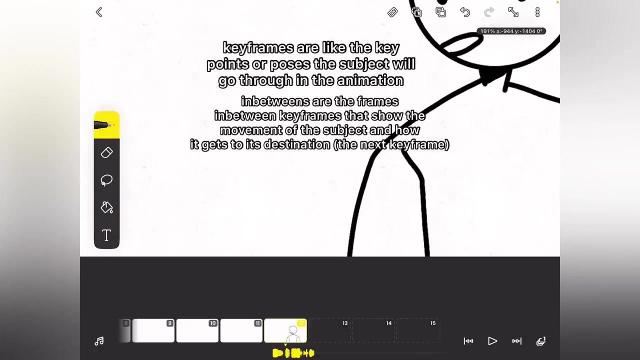 Too thick. Oh, I just realized I had like the wrong background. Well, that's, that's great. That's just great, Anna. And these here are the keyframes that I'm just gonna be drawing first, before I draw the in-betweens. 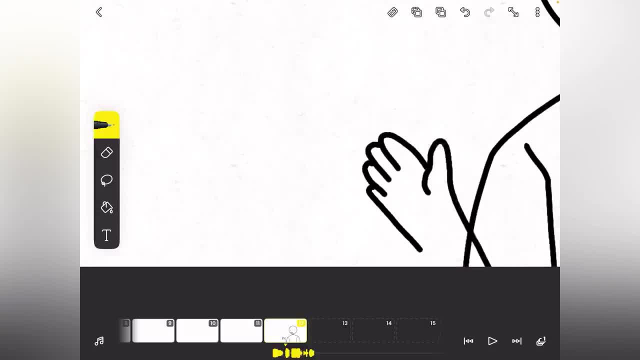 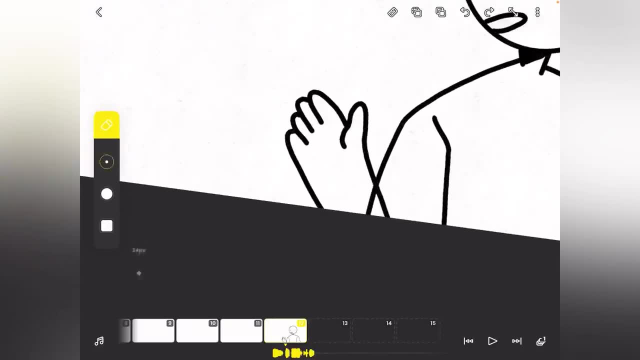 And yes, I know that I can't draw hands. It's, it's like a weakness of mine. I look so weird. Well, that's gonna have to do. Oh, I just realized this is floating off the bottom a bit here. 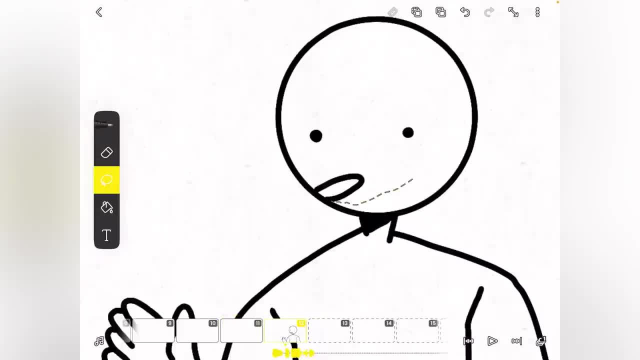 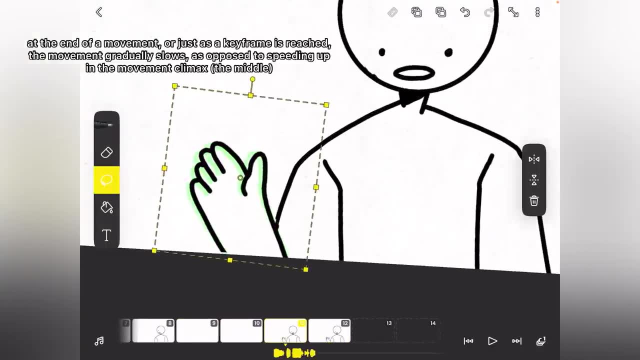 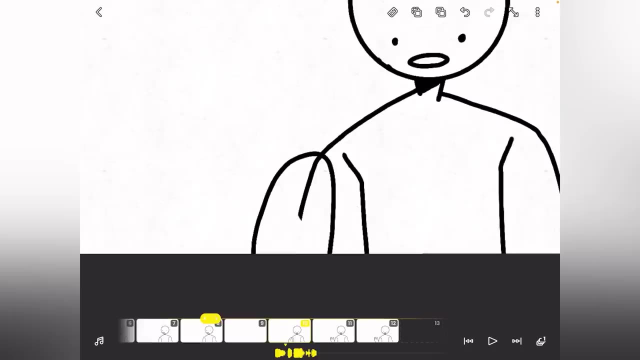 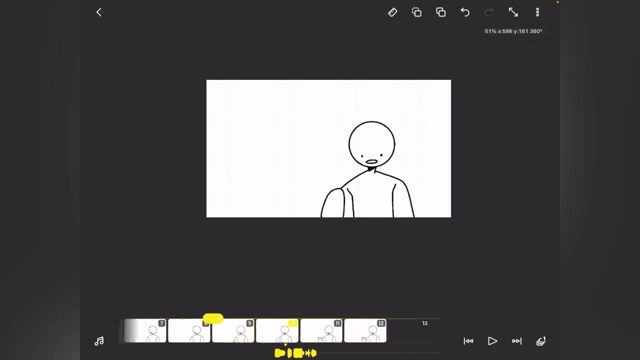 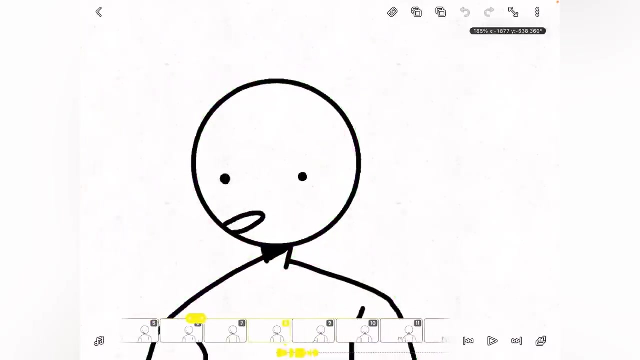 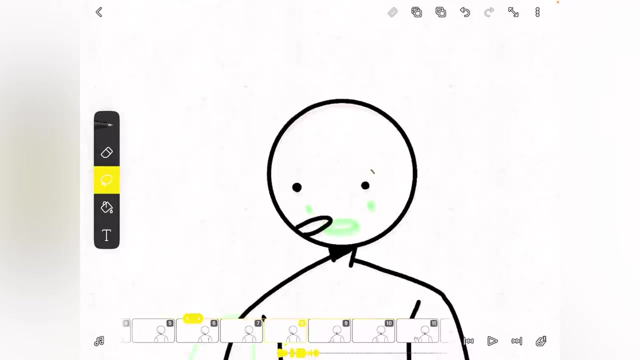 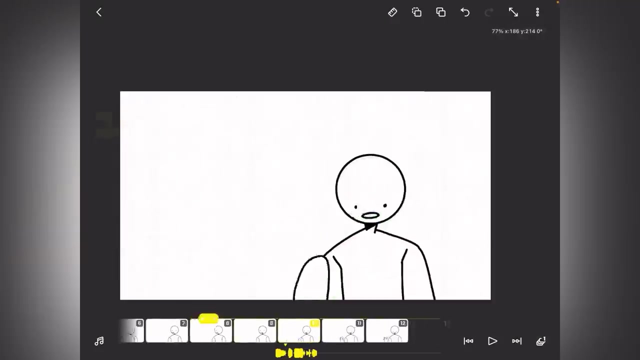 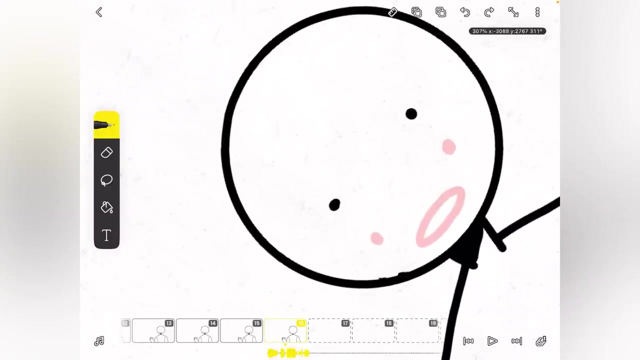 Unacceptable. Wow, Wow, that's great. Now we need to animate the face changing from this to this, Because otherwise it looks very choppy and weird. Wow, Wow, that actually doesn't look so horrible. I cannot draw, Wow. 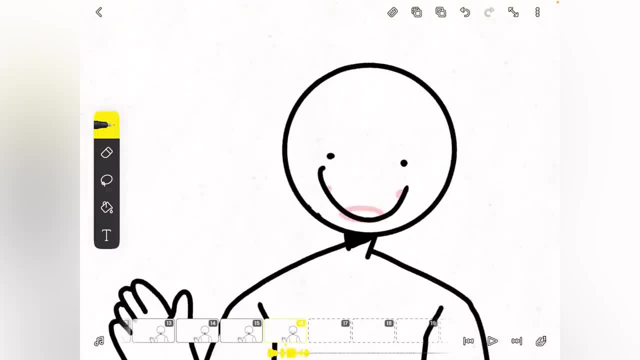 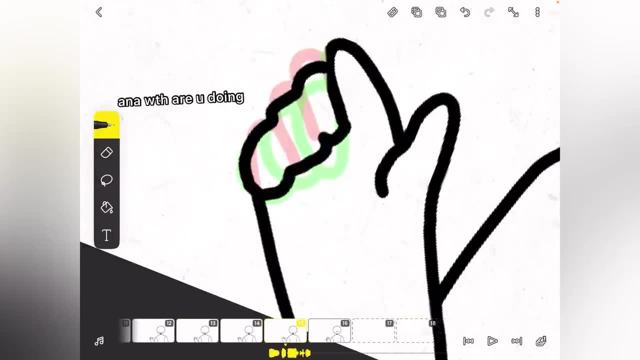 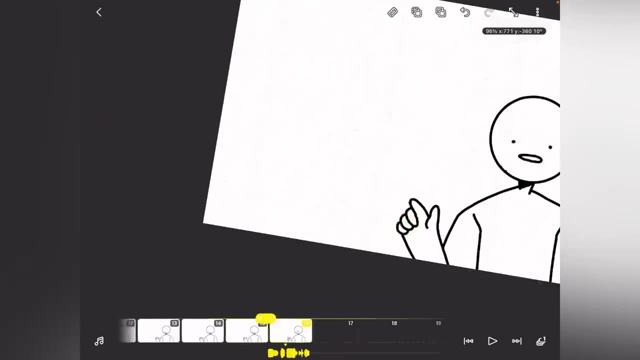 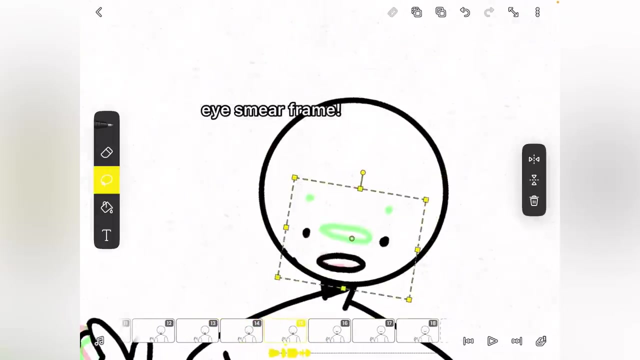 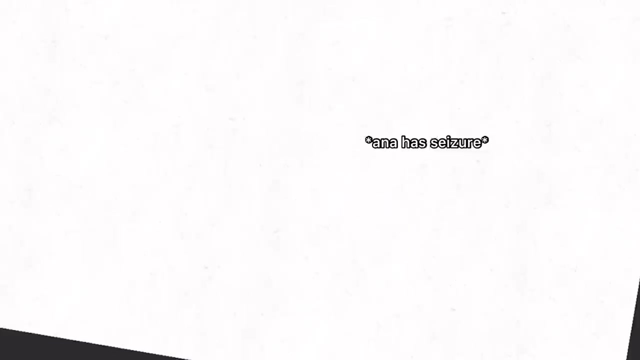 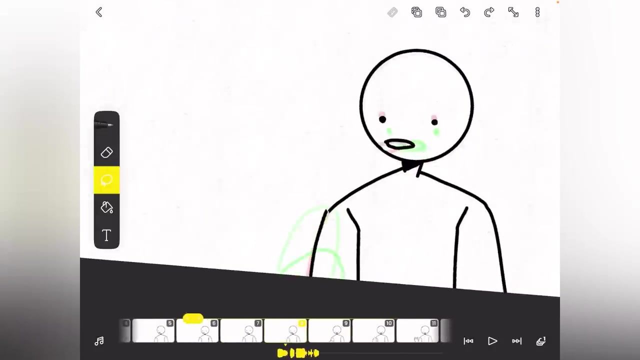 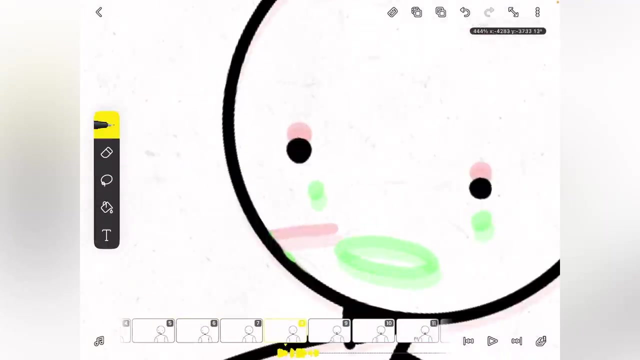 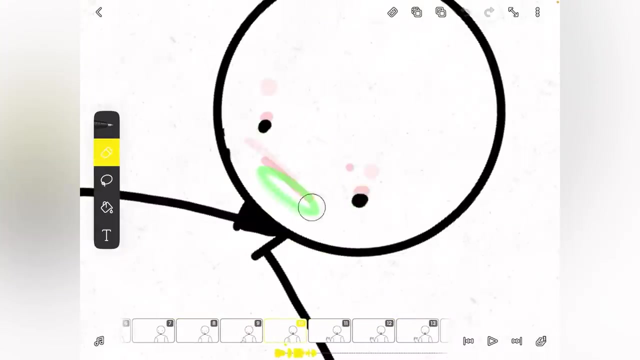 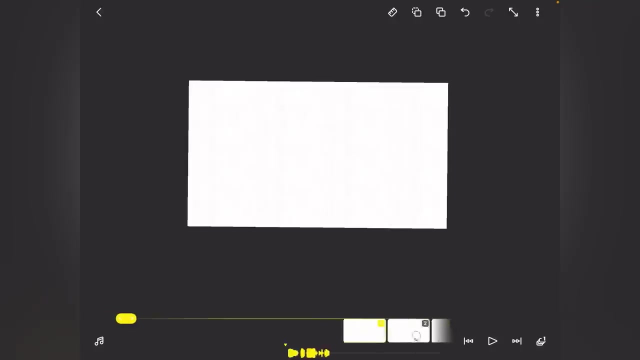 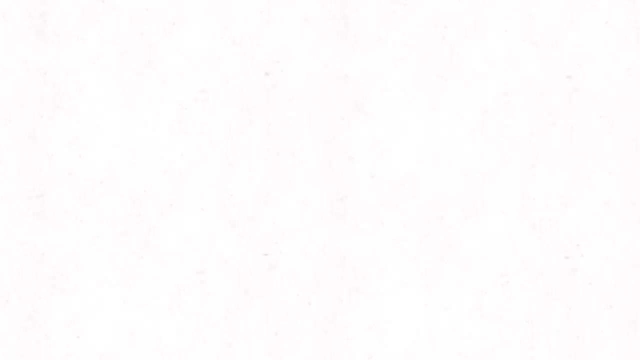 Wow, Yeah, this is this is great. 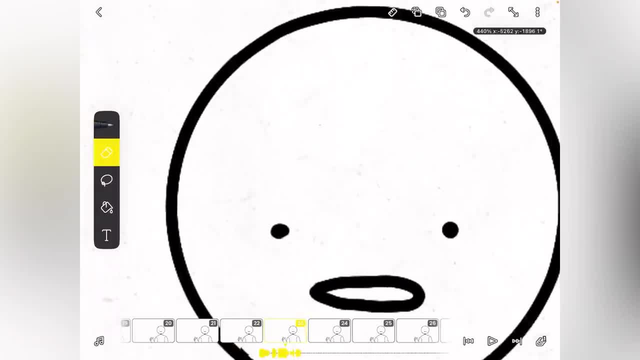 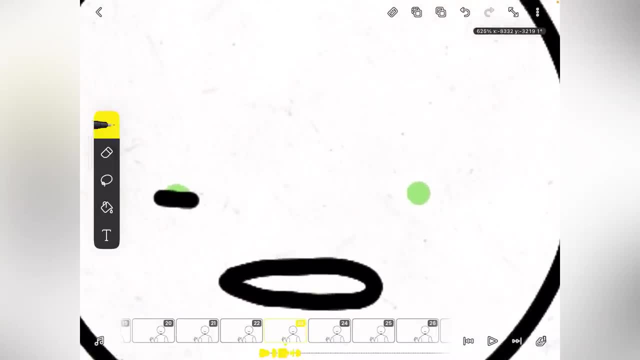 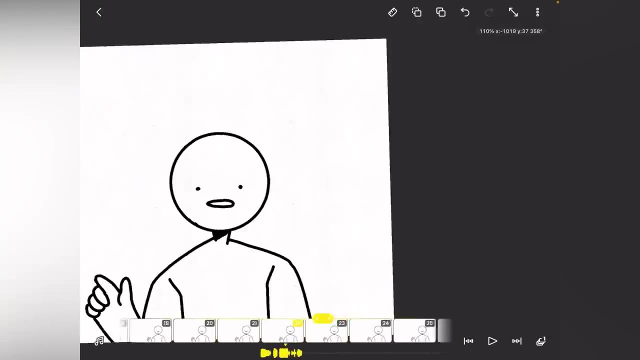 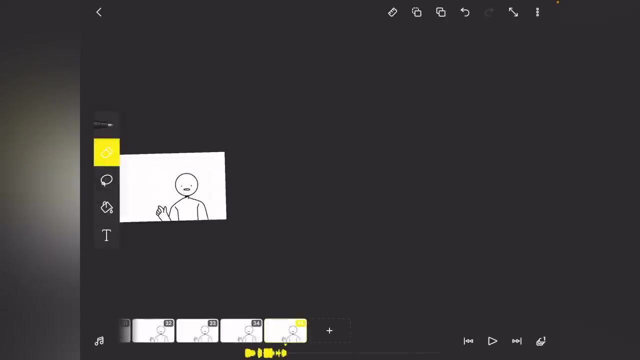 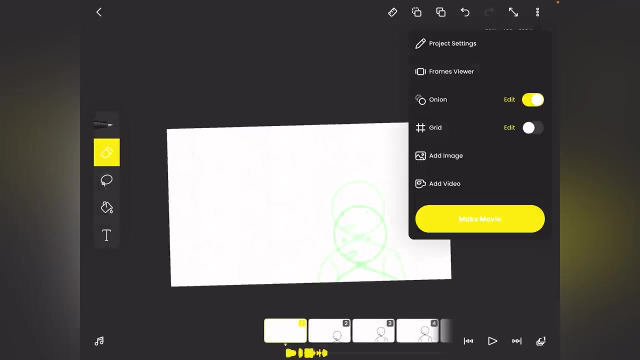 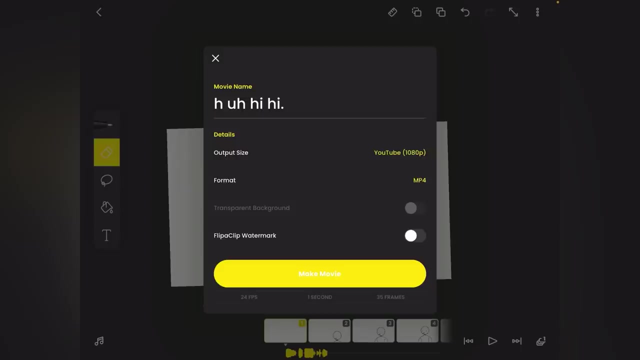 Yeah, that looks really weird, but who cares? um, I like chicken, um, I like chicken, all right. now, as I said, we are going to make a movie and our movie- uh hi, hi- is going to be an mp4 and it's not gonna have a flip a clip. watermark. 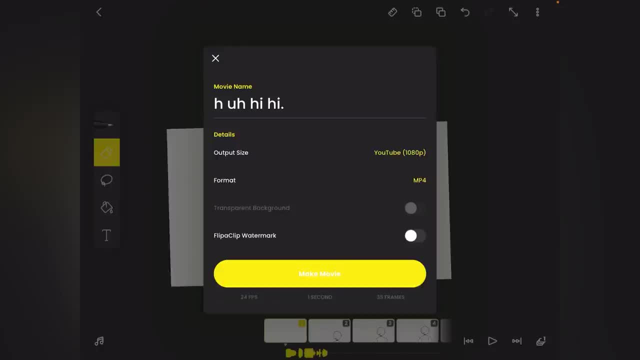 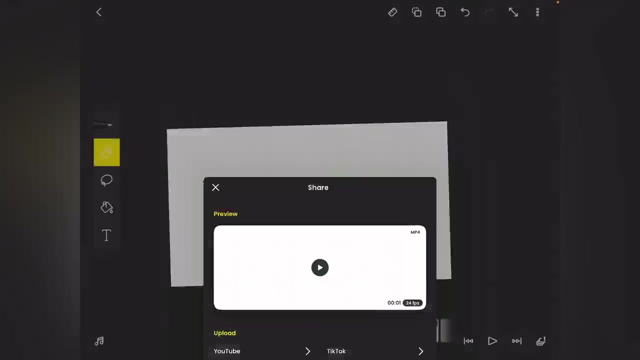 because I paid for the pro version, but if you just downloaded it, you probably haven't, but I recommend doing it. oh, look, it's a whole one second long. okay, we're gonna make the movie. wow, I can save the photos and now you can see the final product. um, I, I like chicken. um, I, I like chicken.